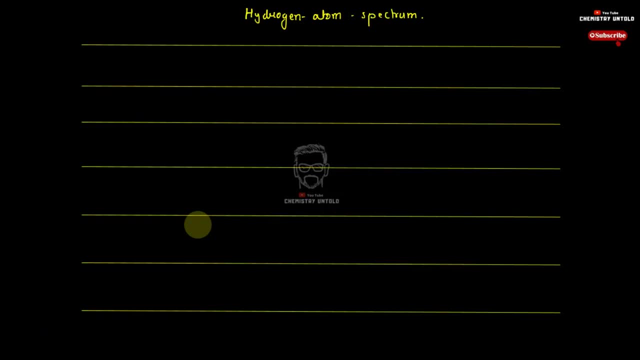 Hey, hello everyone. So in this particular video, let us try to understand hydrogen atom spectrum. Now, this hydrogen atom spectrum is really, really useful. You will be surprised to know that this hydrogen atom spectrum is one of the most important experiment, or I can say, the. 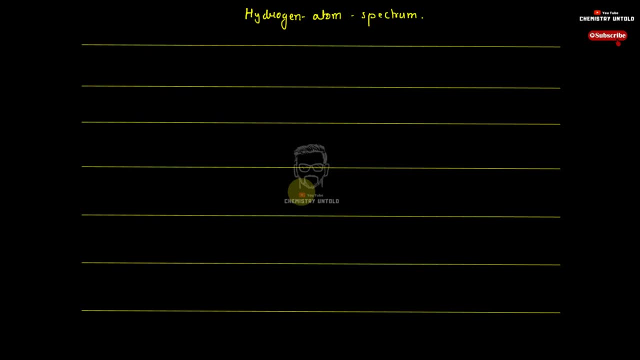 first spectroscopic experiment that led to the discovery of many, many, many important phenomenons in atomic world. Now, before I start with this, well, you should be aware, with few of the things that is, the energy of an electron in a Bohr's model. Energy of an electron in a Bohr's model. 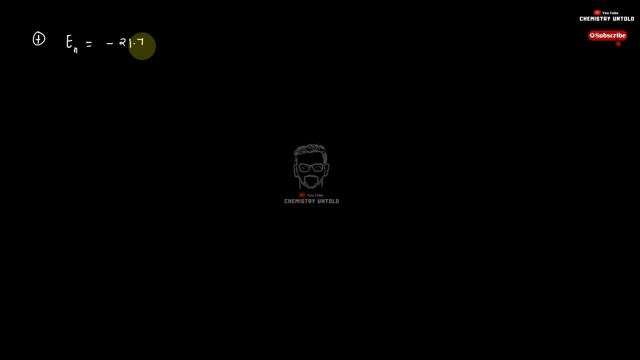 is given by a formula that's minus 21.79 into 10 to the power, minus 19 into z square divided by n square, and this answer will be in joules. Okay, Now, well, how you derive this equation, How you? 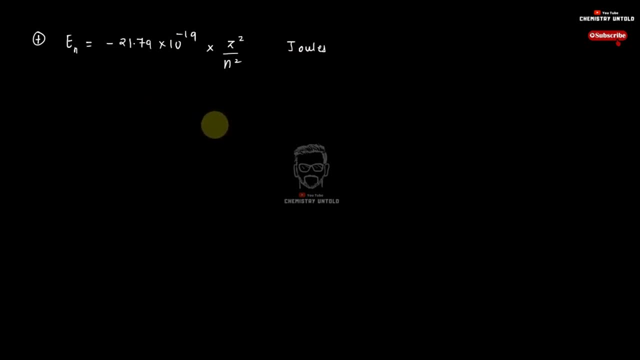 derive this formula. The derivation for this is already given. If you visit my channel, if you visit the video section of my channel, you will find that there's a video in which I have derived the equation, the radius Bohr's- radius Bohr's energy formula. Okay, From there you can just see that, how I derived this equation. Now, 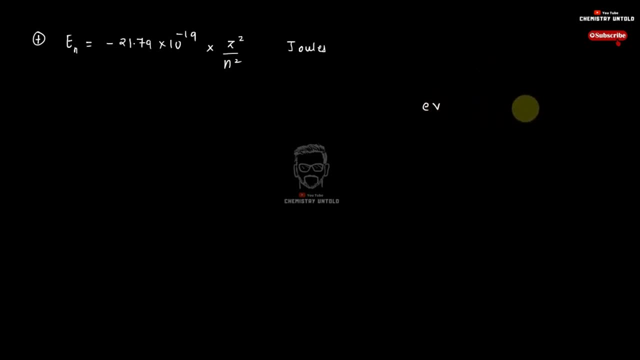 well, there's one more relation: that energy can be either expressed in electron volt and energy can either be expressed in terms of joules. In atomic world we express energy in terms of electron volt. So there's a conversion factor that one electron volt will be equal to 1.6022 into 10 to. 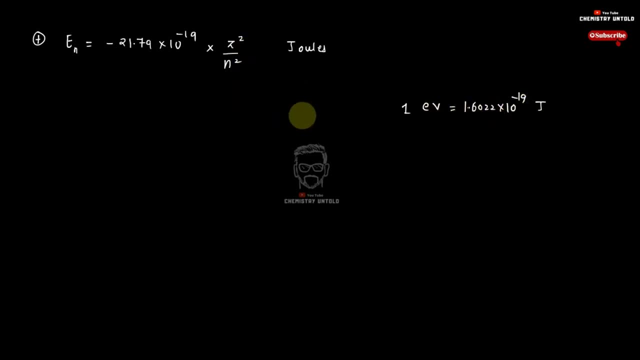 the power minus 19 joules. So using this relation over here, I can convert this joules in electron volt, and the formula that I get will be minus 21.79 multiplied by 10, to the power minus 19 joules. 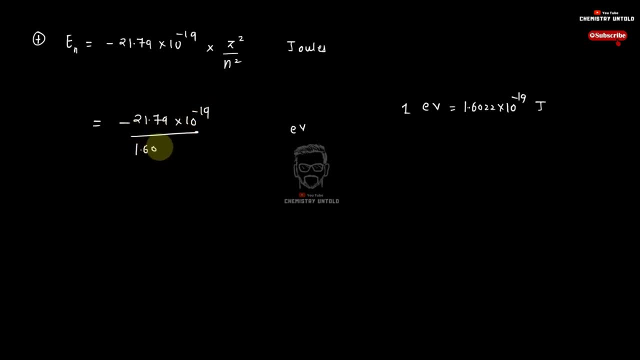 divided by 1.6022 into 10, to the power minus 19, and that will be into z square divided by n square. Well, z over here represents the atomic number. In case of hydrogen it's going to be 1 and n over. 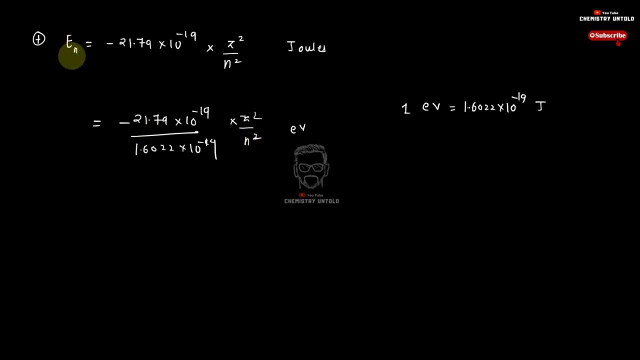 here represents the shell number, Like if you're finding out the energy of an electron in which shell the shell number over there Minus 19, minus 19 over here gets cancelled and the final answer that you get is minus 13.6 into z square divided by n square electron volt. Now this is the formula. 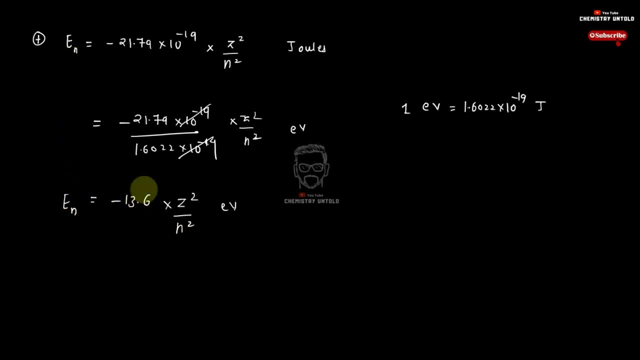 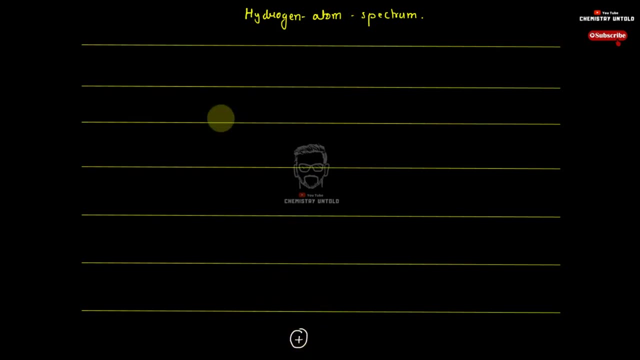 going to use to calculate the energy of any shell in Bohr's model. Now let us start with the first shell over here. Now you must be wondering that hydrogen has got only one single electron there, then how can there be multiple shells present over here? Look for an hydrogen atom, even though the 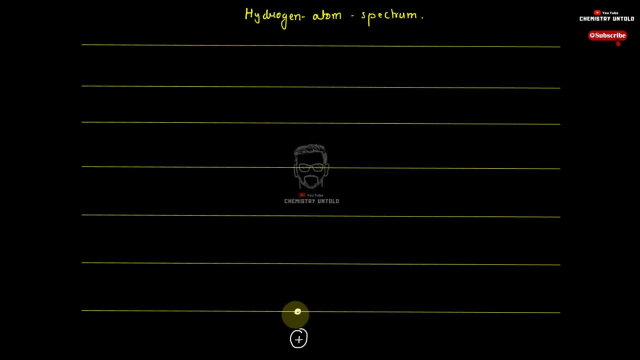 electron will always be present in the first shell, but that does not mean that electron cannot be present apart from this first shell. Before leaving nucleus, the electron can be present at seven different positions and then, probably once it has got enough energy, the electron will be free to. 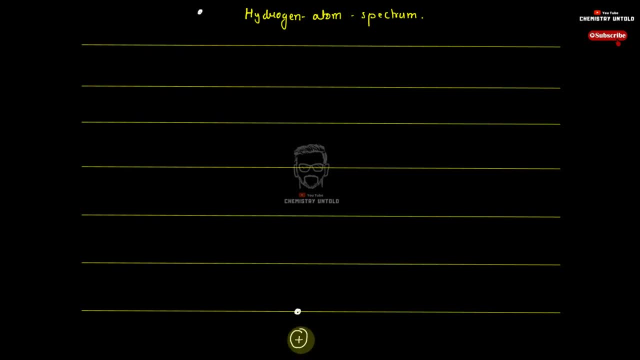 go around and will not be bounded by or will not be under the influence of your proton or your nucleus over there. So, before leaving the first shell, before leaving the sphere of influence of this proton or this nucleus, there are seven different positions where your electron can be. 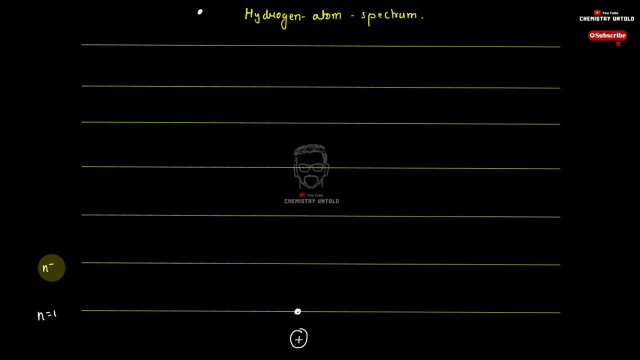 present Accordingly their number: it's n equals to 1, n equals to 2, n equals to 3, n equals to 4, n equals to 5, n equals to 6, n equals to 7.. So there are seven different shells, or seven. 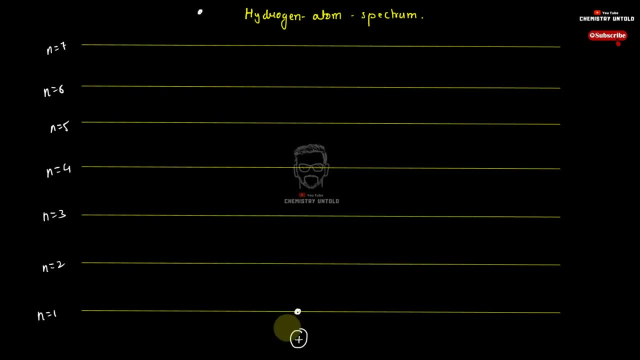 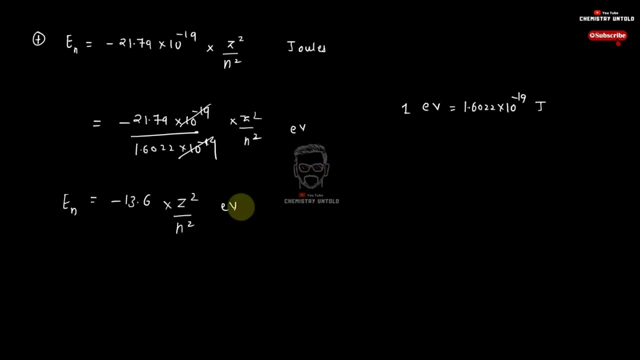 different positions where your electron can be present before leaving your nucleus. Now, the energy of every shell, energy of every shell, can be calculated using the formula which I already mentioned over here. Using this formula, I can calculate the energy of any shell and the 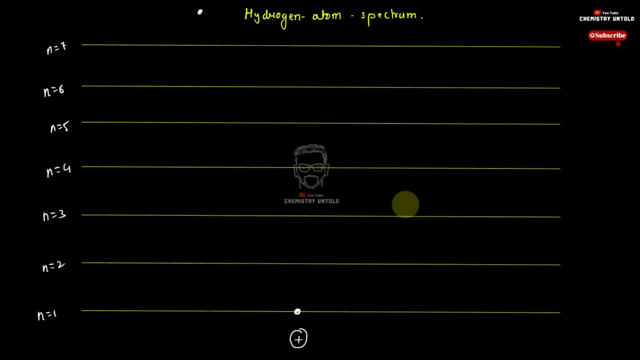 formula that I'm going to use will be in electron volt rather than in joules. So the energy of first shell somewhere comes about to be minus 13.6 electron volt. Energy of the second shell comes out to be minus 3.4 electron volt. It's minus 1.51 electron volt. It's 0.85 minus 0.85 electron volt. 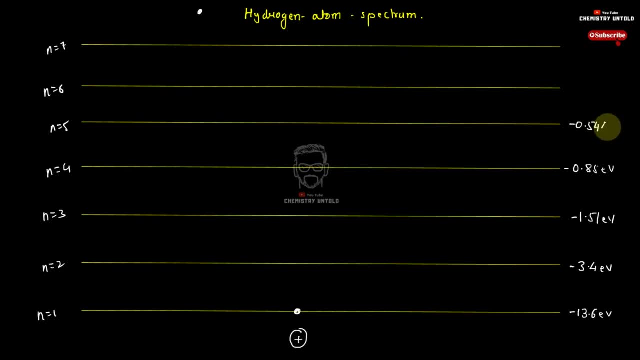 It's going to be minus 0.54 electron volt. It's going to be minus 0.377 electron volt. I have already calculated these values, So you can just even cross verify me if you feel that I may have committed a mistake somewhere. So you just can cross verify. This will be electron volt Now. 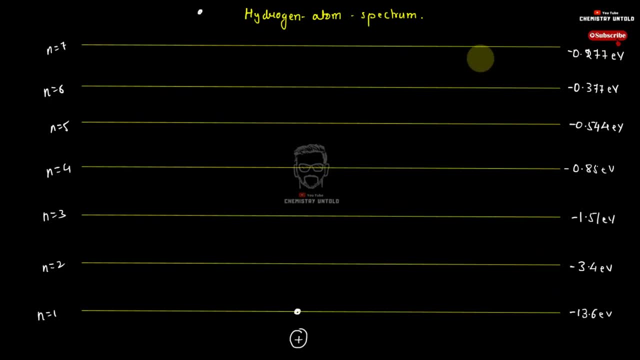 you know, there's a formula again to calculate the difference between energy levels, Like as if I want to calculate the difference between energy shell number 4 and energy shell number 3.. Is there a difference? Yes, Energy at shell number 4 will be higher than the energy at shell number 3.. So 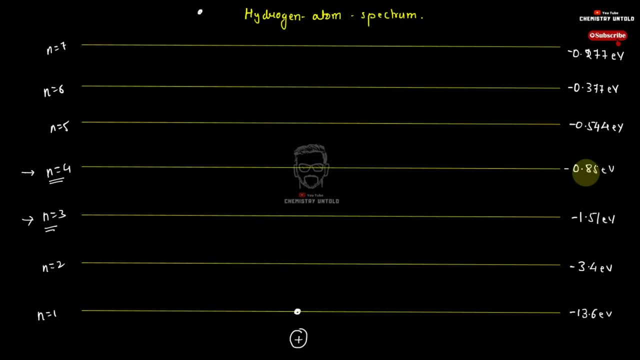 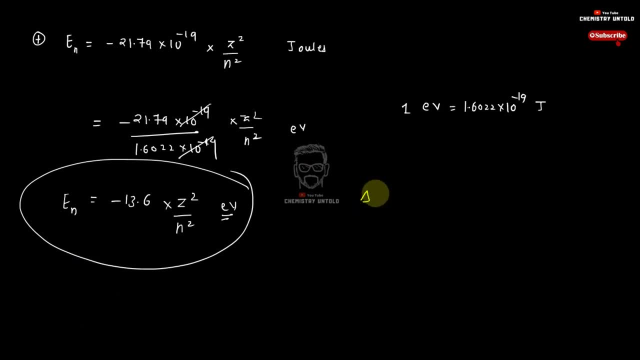 the energy at shell number 3,. the simple reason is, you can see, minus 0.85 is greater than minus 1.51.. Okay, So there's a formula to calculate the difference of energy between any two shell, And that formula is given by delta. E will be equal to 13.6, 13.6 into Z square upon 1 upon. 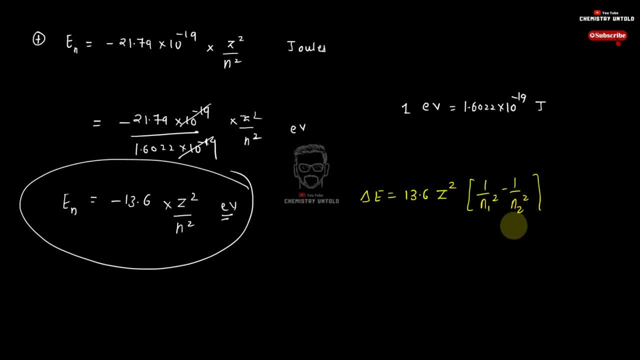 N1 square minus 1 upon N2 square Over here. N2 simply means the higher shell, It simply means the higher shell, And N1 over here simply means the lower shell. Okay, The lower shell. Now over here. this 13.6 can also be- can also be written as R, That's your Rydberg's constant in. 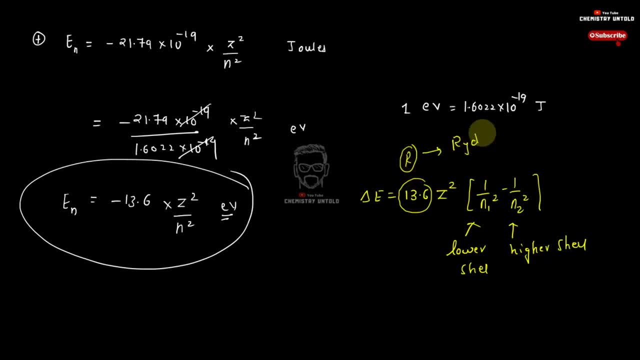 terms of joules, in terms of electron volt. It can also be written as a Rydberg's constant: Rydberg's constant in terms of, in terms of electron volt. So the formula for energy difference between any two level is given by R into Z, square upon, into 1 upon N1, square minus. 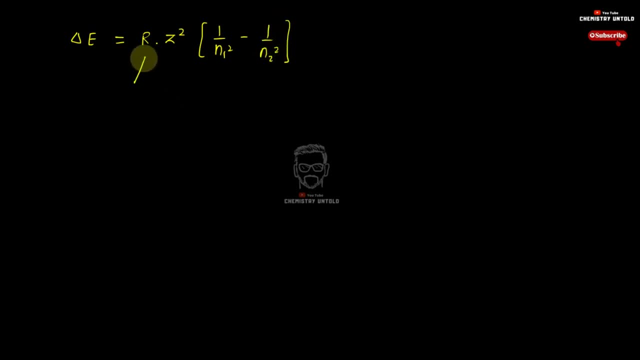 1 upon N2 square. That's the formula which you get Over here. R can either be 20, 21.79 into 10 to the power minus 19 joules, or it may be 13.6 electron volt. Now let me tell you. 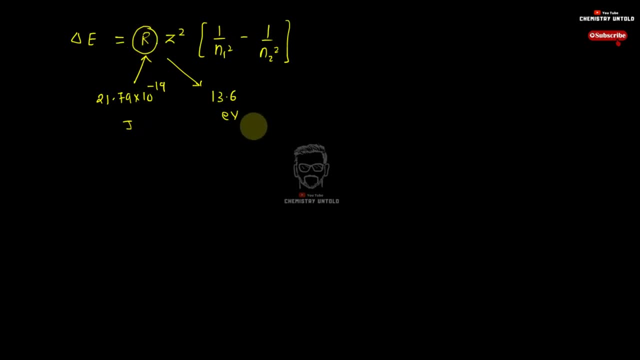 this R over here is Rydberg's constant in terms of joules and electron volt, The value. what do you use? If you use this value, the answer will be in joules. If you use this value, the answer will be: 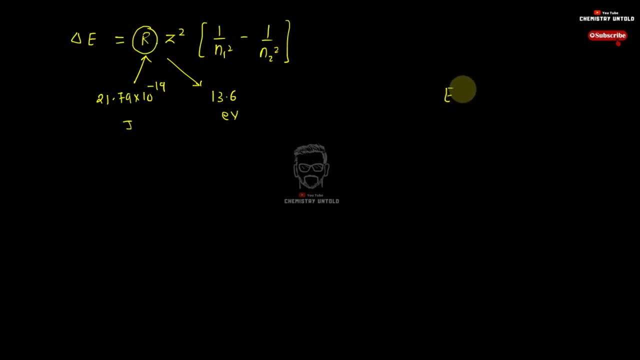 in electron volt. Now there's one more relation that we know: that energy is given by a formula H into mu as well as speed of light, or electromagnetic radiation is given by a formula mu into lambda. Now, over here, R is given by a formula H into mu as well as speed of light or 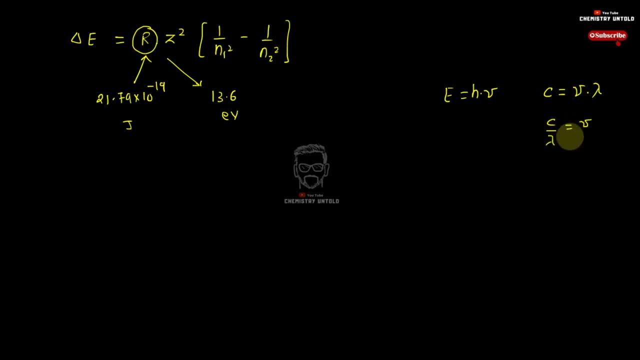 electromagnetic radiation is given by a formula, mu into lambda. Now over here the mu can be replaced by C upon lambda. C upon lambda can be written as mu. Mu is frequency. over here The formula will be: E will be equal to H into C by lambda. 1 upon lambda is again wave number. So 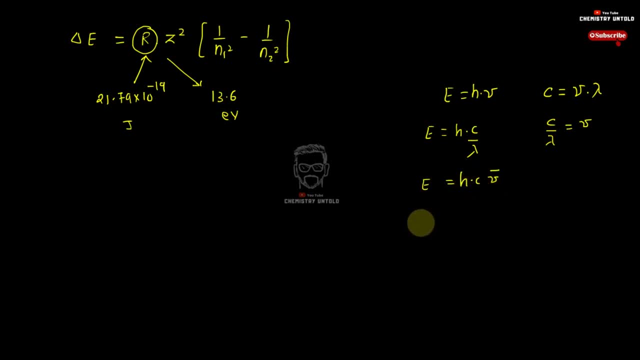 energy will be H into C, into wave number. So can I say wave number will be equal to energy divided by H into C. That's Planck's constant multiplied by speed of light. Over here this is energy Many a times. instead of energy, the people may ask, suppose the energy gap between 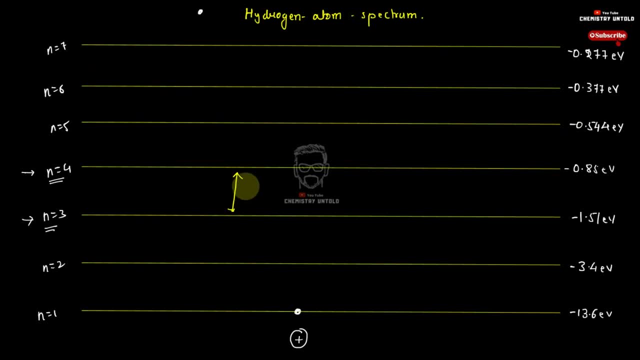 shell number 3 and shell number 4 is equal to energy divided by H into C. So energy will be equal to energy divided by H into C. So energy will be equal to energy divided by H into C. So can you convert that electron volt into frequency? Yes, it can be converted into frequency And the 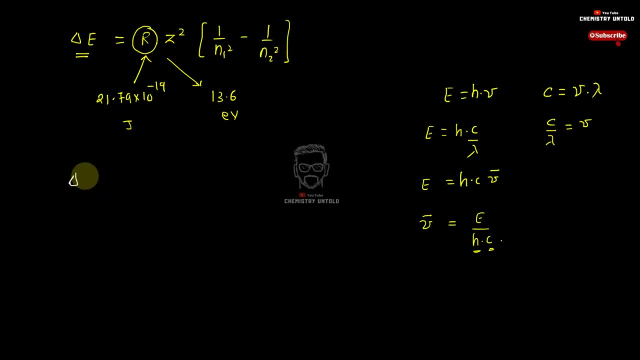 simple conversion unit will be. you just need to divide this energy by H into C, So what you will be getting will be 1 upon lambda. That is nothing but mu bar. So the formula will become this Redberg's constant in terms of joules, or electron volt, divided by H into C. Now, this can be. 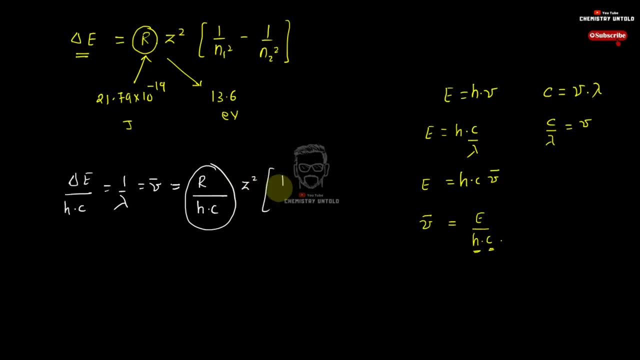 written, as this can be written as N into Z square: bracket 1 upon N1 square minus 3 Joules 1 upon n2 square. now the new value for red box constant in terms of centimeter inverse or meter inverse. it will depend whether you are using the value of h and c in centimeter or meter. 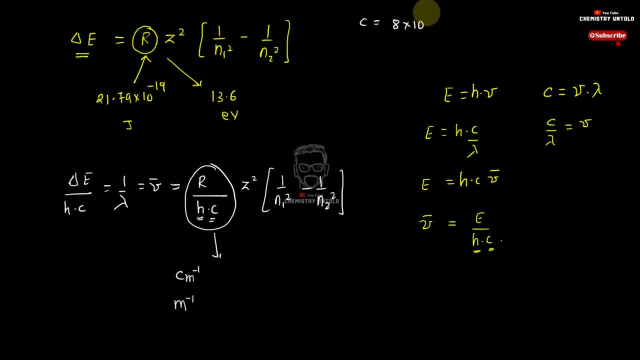 because speed of light. speed of light is given by 8 into 10 to the power- 8 meter per second, or you can even use it in centimeter per second- and the value of h is given by 6.626 into 10 to the power. 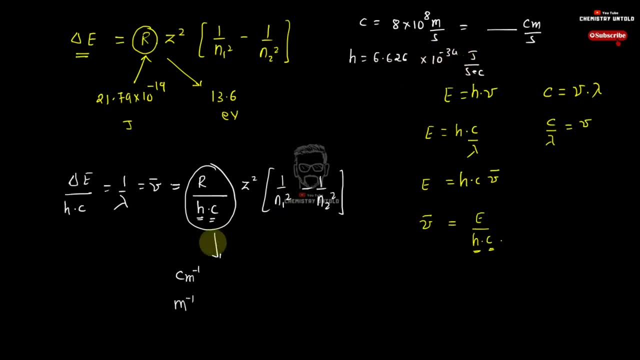 minus 34 joules second. now, depending upon what value you are using, either you are using it in meter per second, or joule per second, or centimeter. the value of this new term, that's r divided by h into c, can have different units, can have different value. that's either in centimeter or meter inverse. 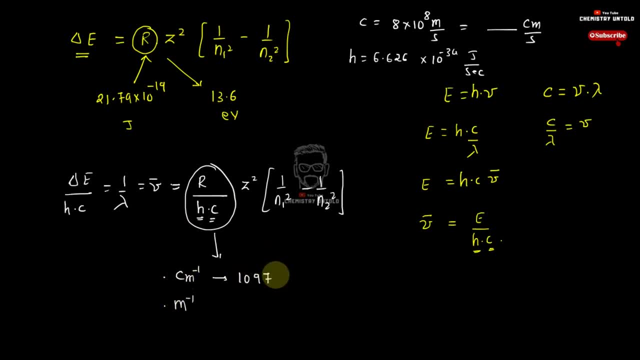 in centimeter. it is written as 109743 centimeter inverse. now, accordingly, you can convert it into meter inverse. okay, the conversion unit is quite simple. so this new thing is also called as red box constant. it's r divided by h into c, but this red book constant will be in terms of centimeter. 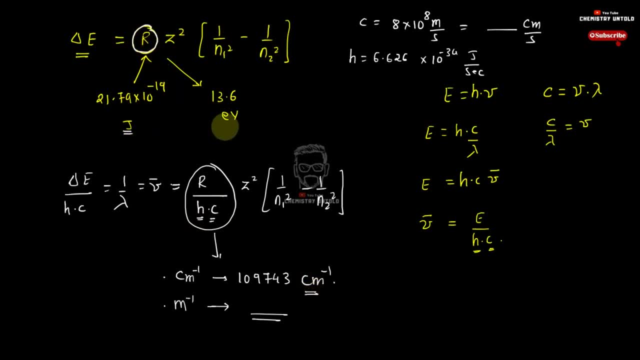 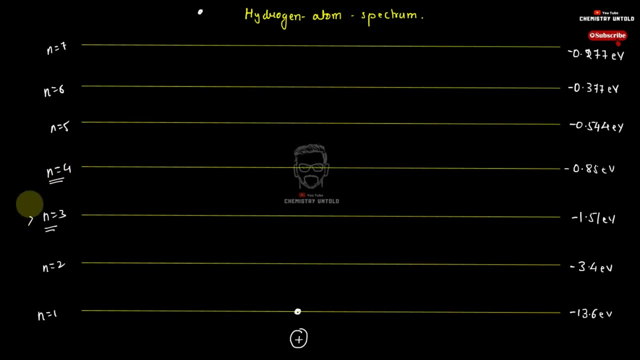 inverse over here. the red book constant is in terms of joules or electron, one volt. now, with the help of this, i have already calculated the energy difference. i have calculated the energy difference between the shells present over here. the energy difference comes out to be 10.2 electron volts: 13.6 and 3.4. so the difference will be 10.2. the difference between over here. 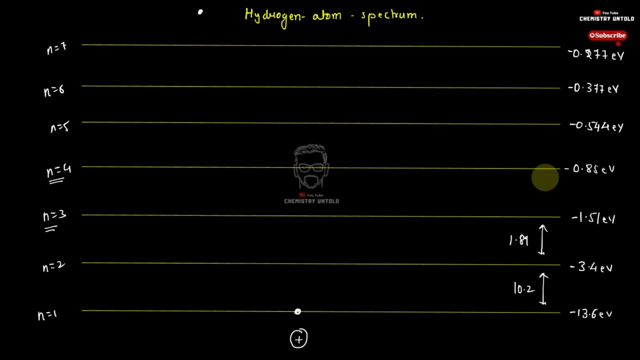 comes out to be 1.89- 1.89. the difference over here comes out to be: the energy difference between two shell comes out to be 0.66- 0.66. the energy difference over here comes out to be 0.306, 3.0. 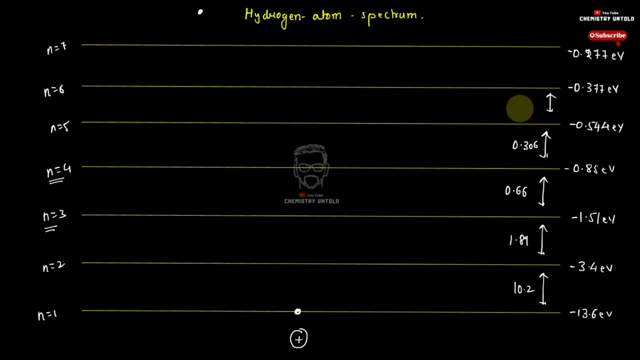 0.306, the energy difference over here comes out to be 0.167. if you look carefully, the difference of energy between two shell is continuously decreasing and it's an exponential decrement. okay, it's an exponential, not a linear decrement. over here, the energy difference between two 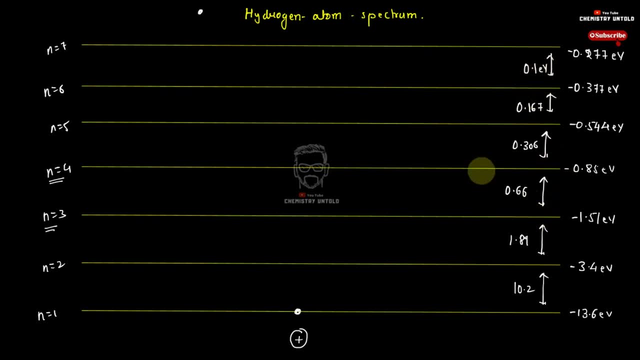 shell comes out to be 0.1 electron volt. now make sure, all the values over here- i don't need to mention all the values over here- are in electron volt. now what is the use of doing all these things like? why are we doing all this thing? well, the simple. 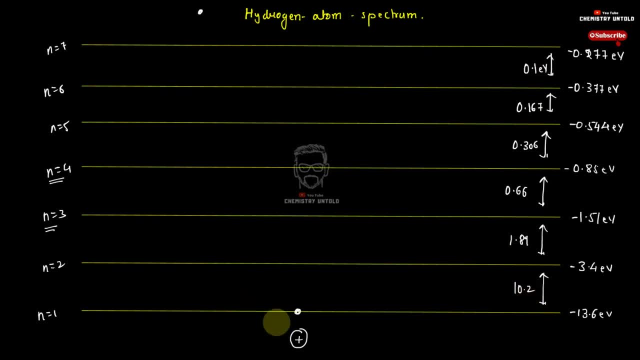 use for doing all this thing is suppose an electron which was initially present in your first shell- that's a ground level- absorbs some amount of energy, and it may be present in any higher shell if your electron, which was present in first shell, absorbs some amount of energy. 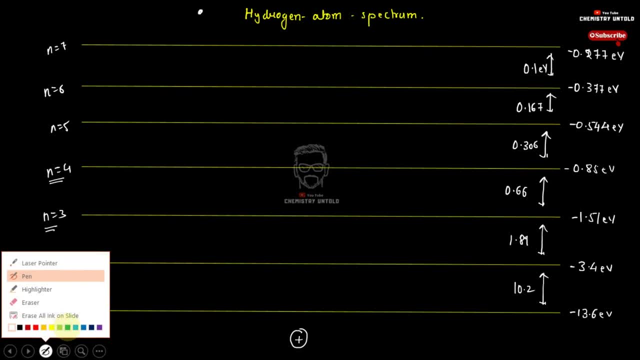 and is present in any of the higher shell apart from your first shell, it may be present over here, it may be present over here. it may be present over here, over here, over here or over here, over here now, if your electron, which has absorbed some amount of energy and it is present in the 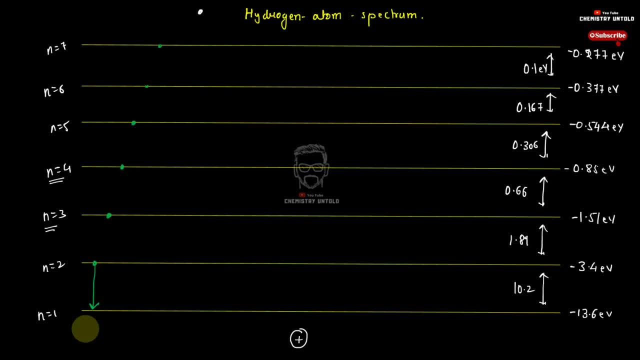 second shell again fall back to first shell. so obviously it's going to emit a certain amount of energy and that energy will be equal to 10.2 electron volts. let me write it over here: 10.2 electron volt. so i don't need to mention electron volt again and again. okay, so the energy, if your 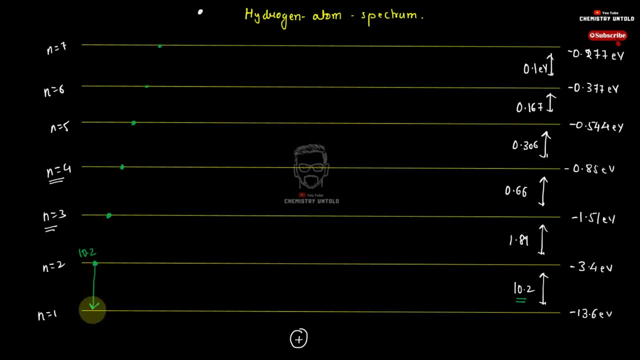 electron jumps from second shell and comes back to the first shell, it is going to emit an amount of energy that will be equal to 10.2. okay, 10.2 now. similarly, if an electron which was present at third shell, if it comes back to first shell now, you must be wondering why it's coming to first. 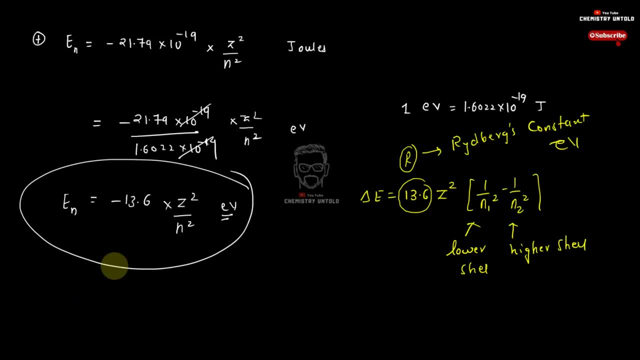 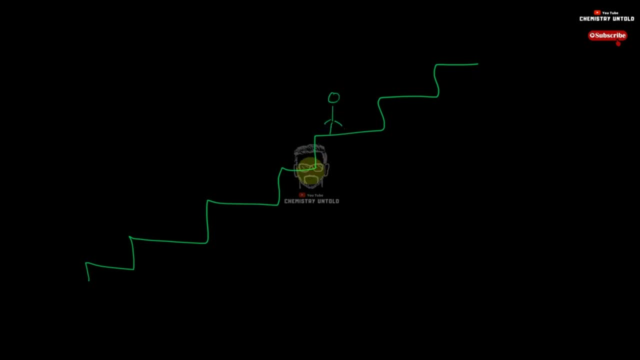 shell, it may also come to the second shell. now i can explain you this in this way. let me raise it out: suppose there are stairs, there are multiple stairs- and a person is standing over here. a person is standing over here and he has got a marble. he's got a marble or a stone in his hand, and if he 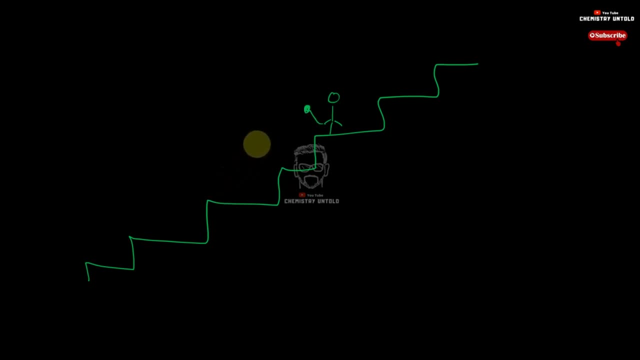 throws that stone. so how many possibilities are there that? in how many different ways the stone can reach the lowest level? it can reach the lowest level. there are many. either it may directly throw it over here, it may throw it by step by step, step by step, step by step, or it may throw it in this. 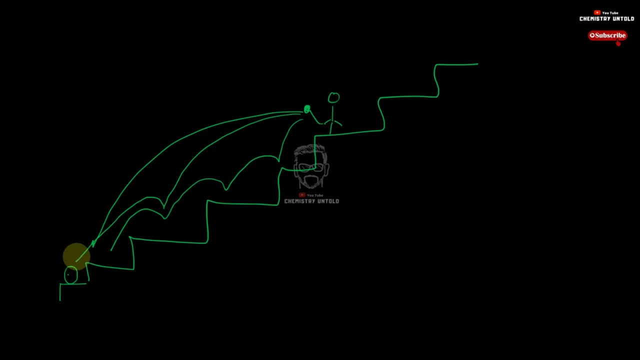 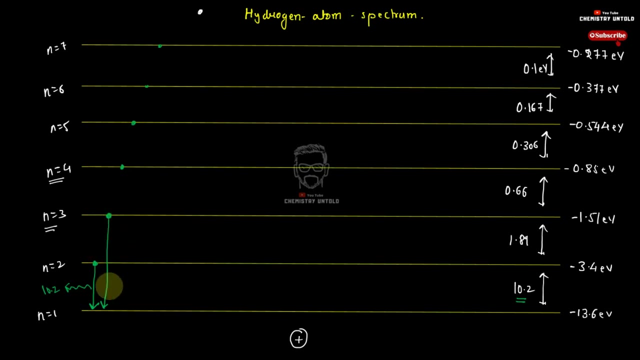 way that it reaches the, the second last shell, and then again it goes to the last shell. so there are many different possibilities. similarly, if an electron is present at shell number three, it may return back to its ground state by different ways. one of the possibilities is that if an electron is present at shell number three, it may return back to its return back to its ground state by different ways. one of the possibilities is that if an electron is present at shell number three, it may return back to its ground state by different ways. one of the possibilities is that if an electron is present at shell number three, it may 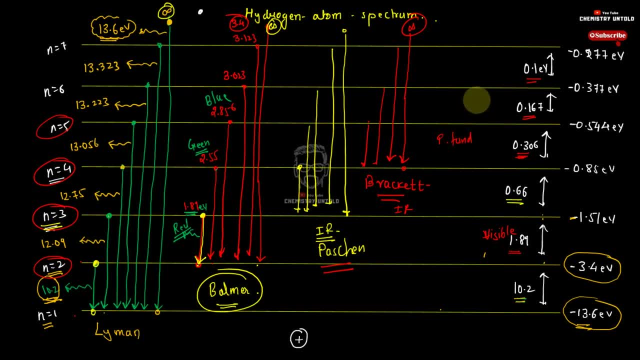 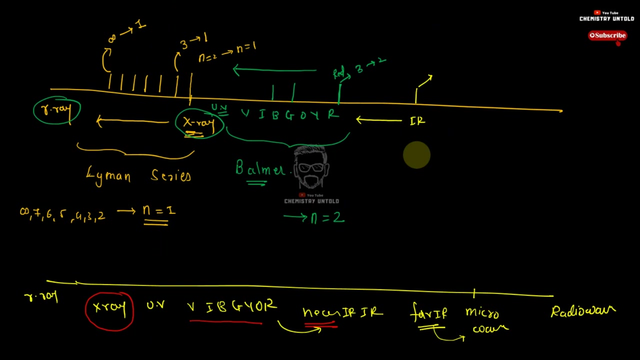 return back to its ground state by different ways. one of the possibilities is that if an electron is present at shell number three, it may. there will be four transition, there will be three transition and there are only two transition which are possible for the this hum free region. okay, my electron is present at any of the higher shell. 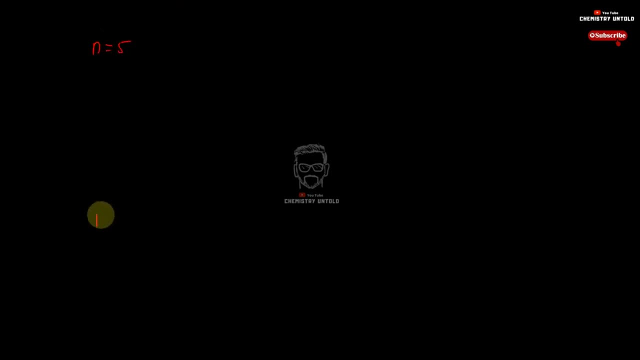 let us say, if it's present at n equals to phi and it's going to return back to n equals to one, so by how many different transitions can it come back to n equals to one? i hope you got my question that if it's coming from n equals to phi to n equals to one, just take an example, it's your. 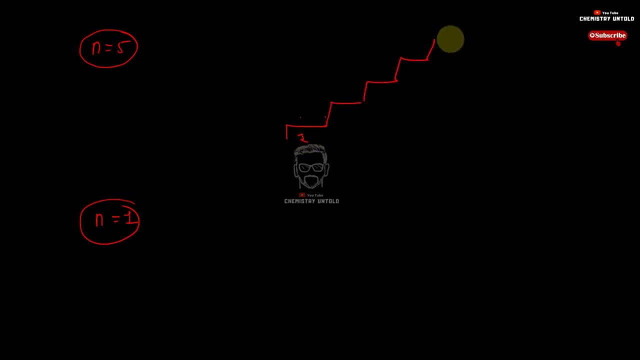 first stair, then you've got a second stair, third, fourth and fifth. now you are standing at stair number fifth. you want to come down. how many possible ways are there for you to return? the first possible transition can be this: directly coming from there to this, or it may be like 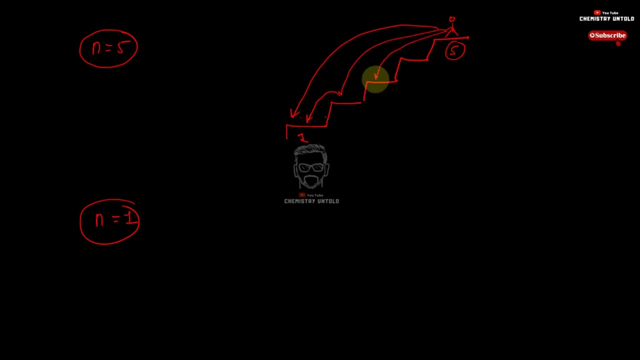 coming to this and then jumping over here, then coming to this, then jumping over here, or coming to this, then this and then this. how many possible transitions are there? how many different spectral lines can be obtained? because every transition is a new, different spectral line. so the formula: 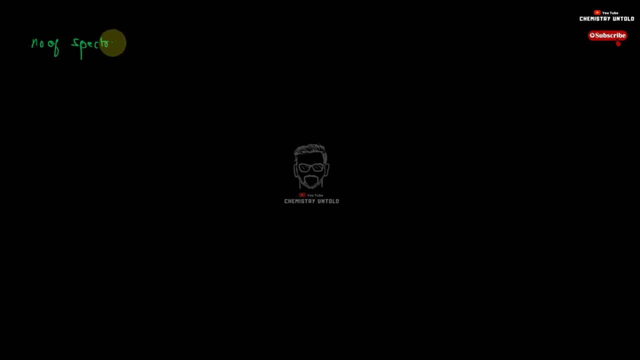 for number of spectral lines. number of spectral lines will be given by n2 minus n1. n2 minus n1 plus one whole divided by four. two over here. n2 is higher shell, n1 is lower shell. in case of this transition, that is, n equals to phi to n equals to one. that's a lyman transition, starting from fifth ending on. 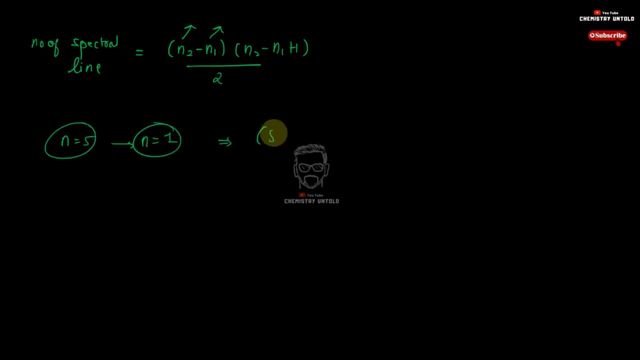 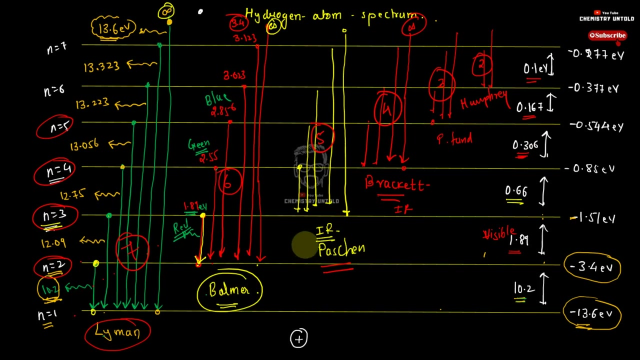 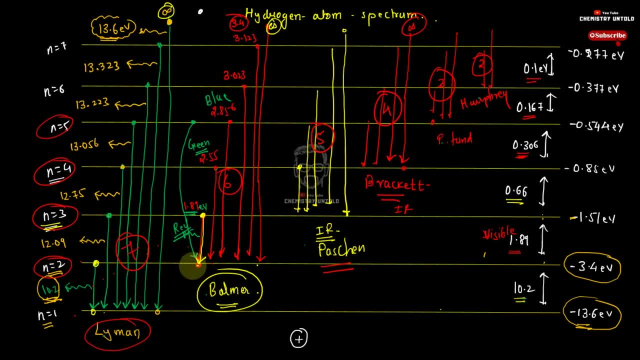 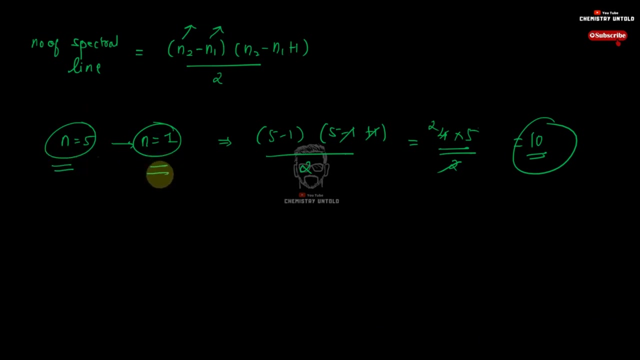 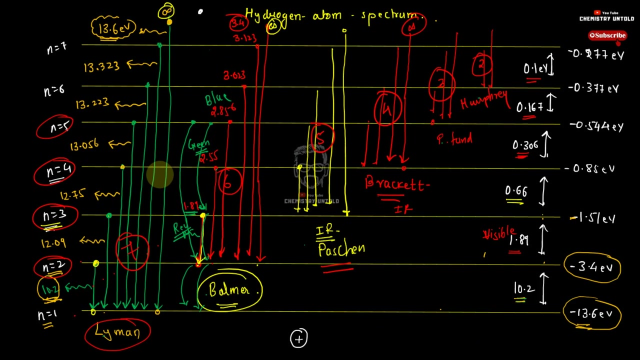 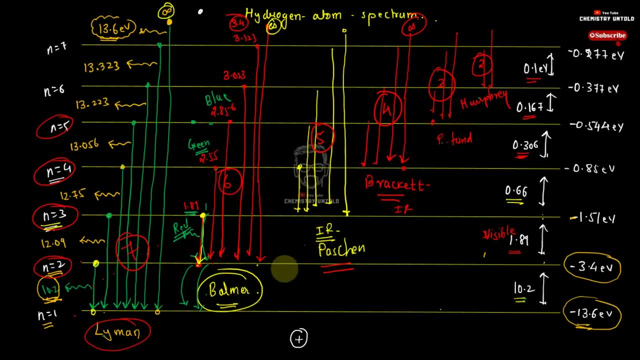 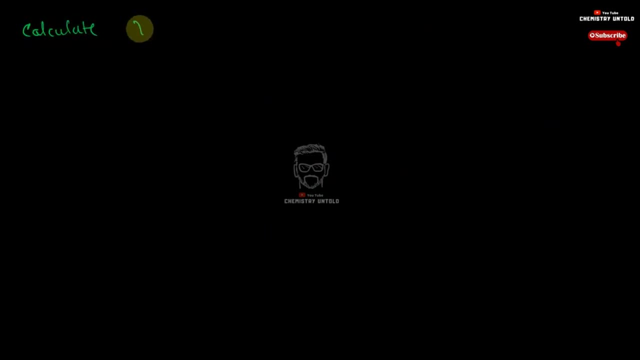 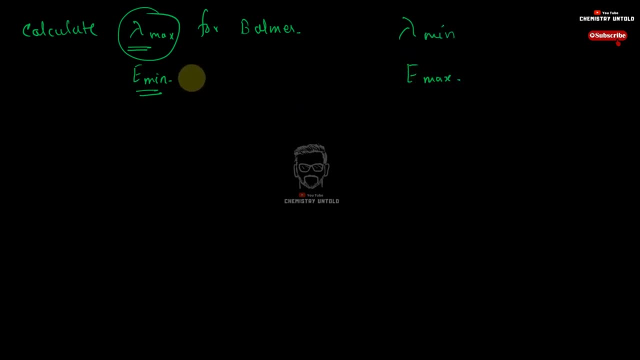 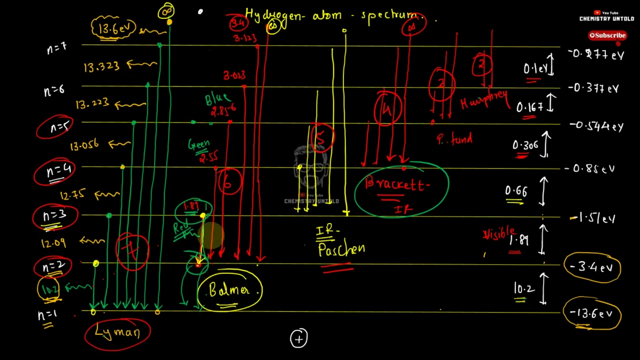 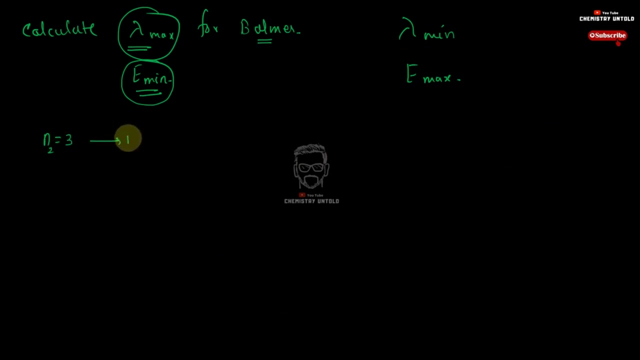 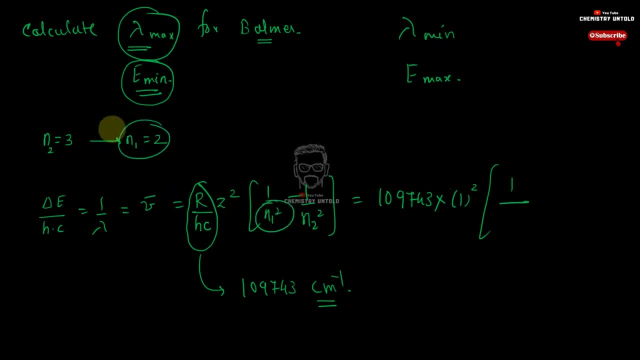 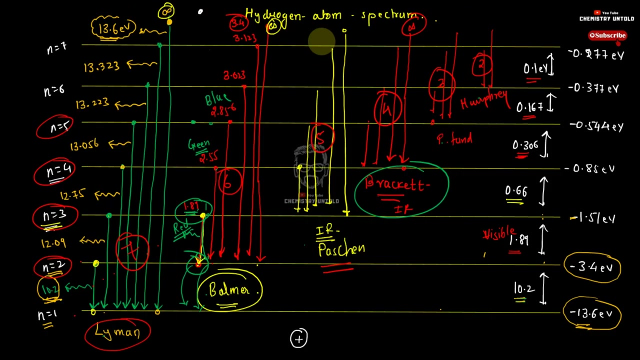 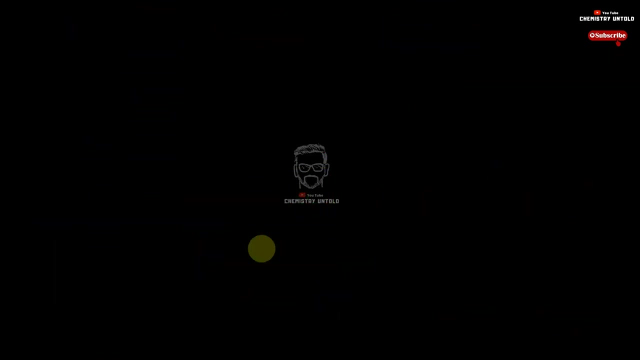 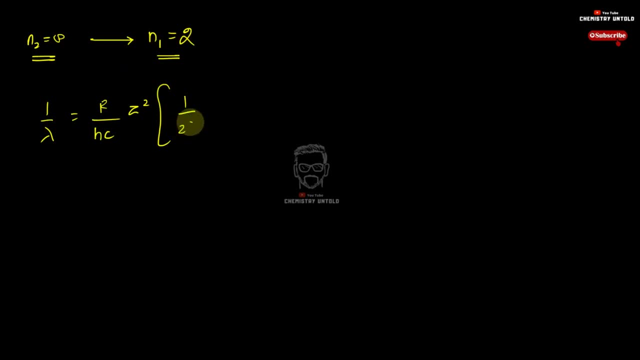 z square, bracket 1 upon n1 square, that's your 2 square minus 1 upon infinity square. okay, 1 upon infinity square. you are trying to calculate lambda minimum, that is, energy maximum. and energy maximum for balmer series will be from infinity to second shell. okay, so this is 109743. this term will get. 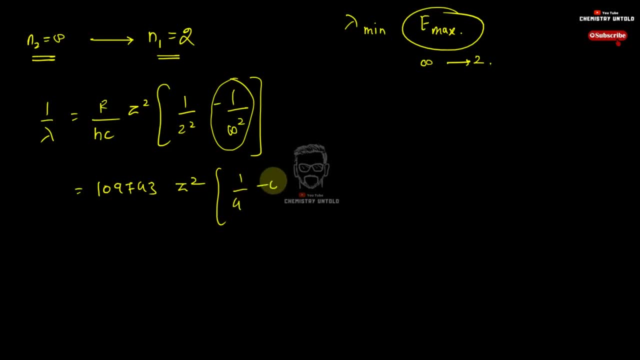 converted to 0, so bracket 1 upon 4 minus 0, just solve it out. z value over here will be 1, so 109743 multiplied by 1 by 4, whatever will be, the answer will be centimeter inverse, because it's 1 upon. 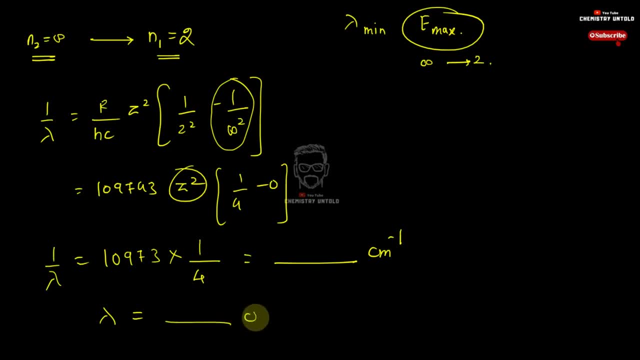 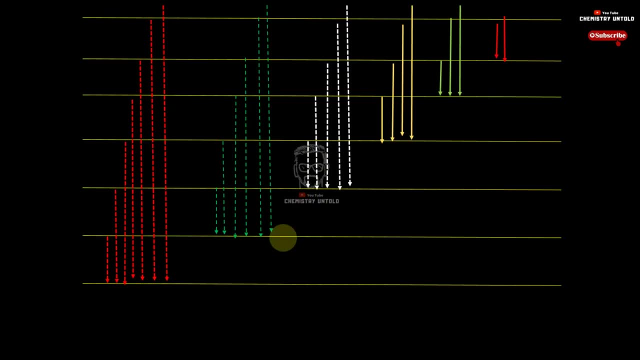 lambda later on. you can convert it, you can inverse it. what you will be getting will be centimeter. convert to nanometer or picometer, as per the question. whatever is asking the question, okay, so i hope. many a times i have seen students finding it difficult to understand hydrogen atom. 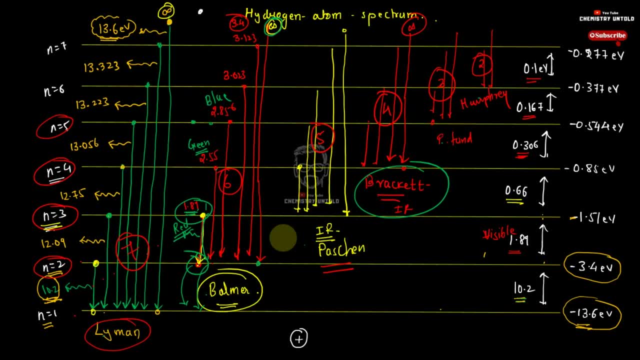 spectrum. this long video where i have discussed in detail the hydrogen atom spectrum is quite enough for you people to solve any question that will be asked in your competitive exam. you now the last thing that i want to ask you is: in this entire hydrogen atom spectrum, entire hydrogen. 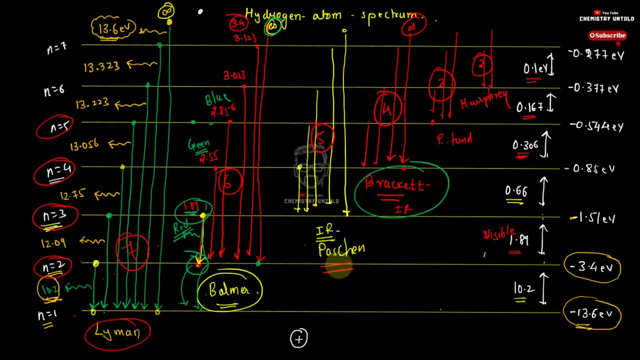 atom spectrum, which will be the lowest energy transition. i'm not asking about any particular series, i'm asking: in this entire hydrogen spectrum, the lowest possible transition will be from infinity to seventh shell. look this transition, look, the difference of energy is decreasing. so this transition from infinity to seventh shell will be the lowest possible, lowest energy. 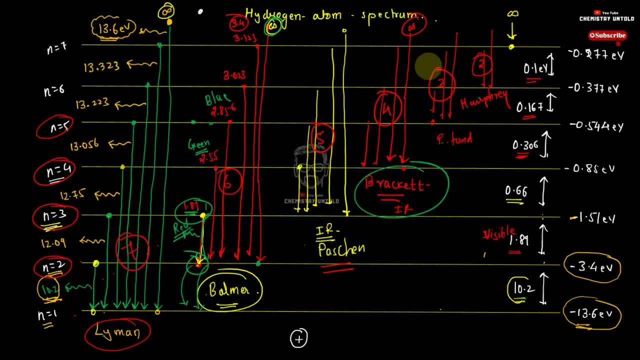 transition in this entire hydrogen spectrum and the highest energy transition and this entire spectrum will be from infinity to the first shell. so the highest energy transition in entire spectrum and the lowest energy transition in entire spectrum. also the highest and lowest energy transition in particular series. you just have to remember these concept and then you can solve any. 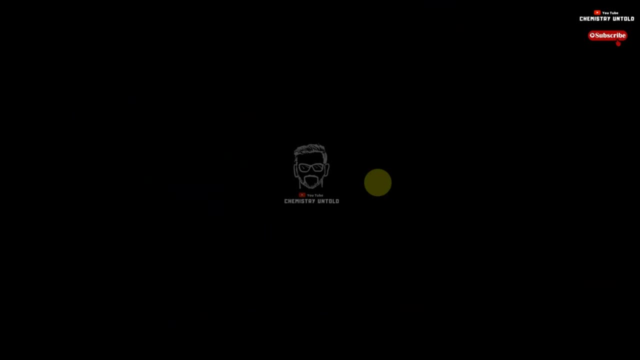 any question as well, as you just need to buy hard all these formulas, the values in case. if you like this video, please do hit that like button and i'll see you in the next one like button. okay, hit that like button and do consider subscribing my channel. for more such videos. till then, bye, bye, take care and god bless you.